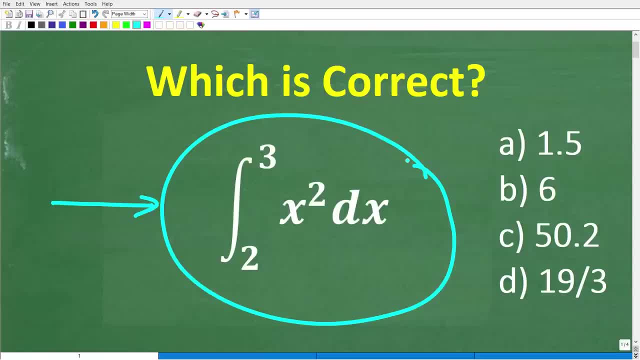 So I'm going to explain this calculus problem in such a way where pretty much anyone will be able to understand it and, more importantly, have an appreciation for calculus and why we need it. But before I get into all of that, for those of you that do know some calculus- or maybe you took this many years ago, or took calculus you know 20,, 30,, 40 years ago- let's see if you can remember how to do this simple calculus problem. 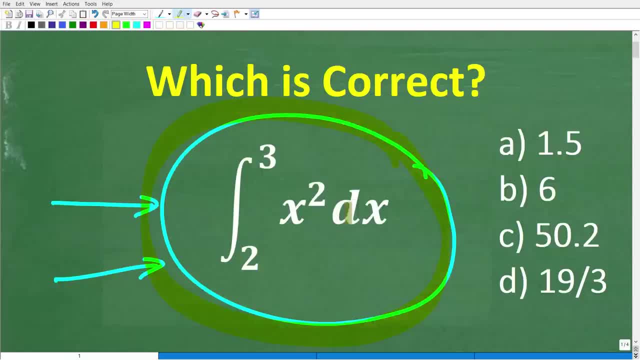 All right, so I'm not going to tell you what it is, but the answer to this problem is over here. So A is 1.5, B is 6, C is 50.2, and D is 19 over 3.. 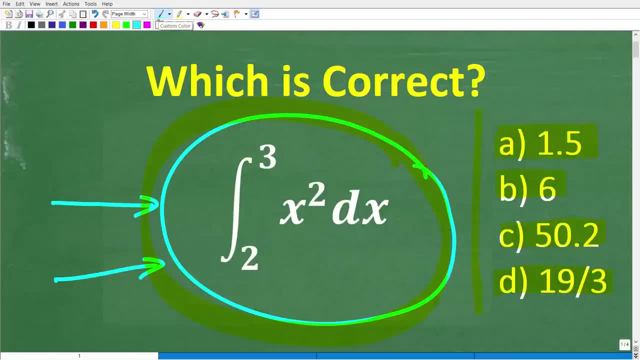 All right now, feel free to use a calculator, but if you can figure this out, go ahead and put your answer into the comment section. I'll share the correct answer in just one second. Then, of course, I'm going to explain this calculus problem- how to do this calculus problem- in such a way where pretty much anyone can understand. 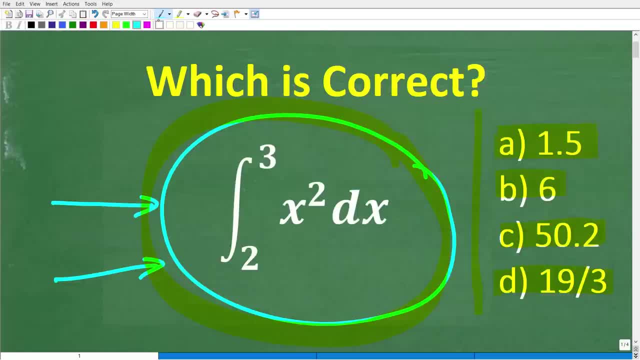 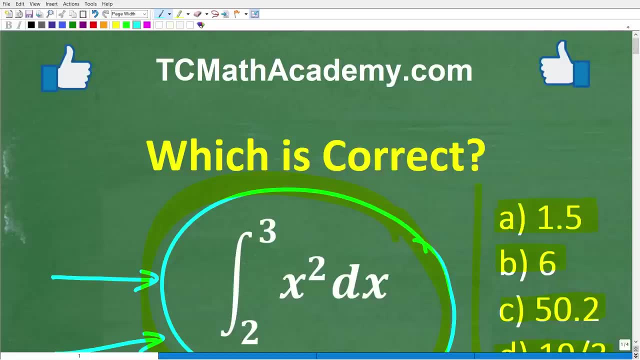 And, more importantly, where everyone can understand And really have a good sense of why calculus is so awesome. But before we get started, let me quickly introduce myself. My name is John and I have been teaching middle and high school math for decades. 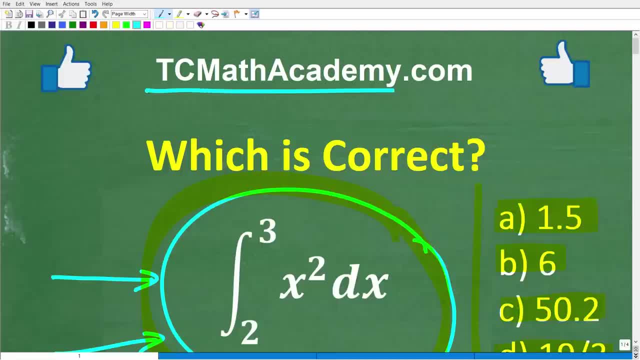 And if you need help learning math, check out my math help program at tcmathacademycom. You can find a link to that in the description below. And if this video helps you out or if you just enjoy this content, make sure to like and subscribe, as that definitely helps me out. 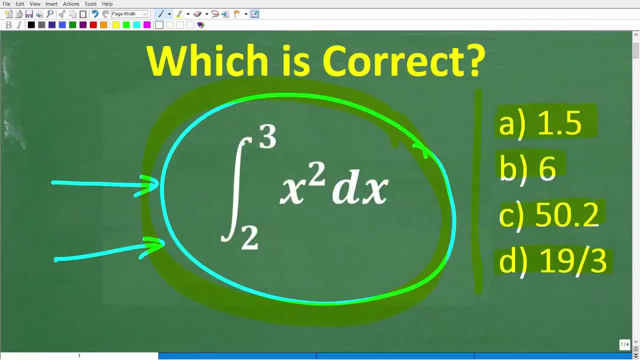 All right. so what we have, What we have here, is an integral problem. That's what this little crazy symbol looks like right here. So we have an integral from 2 to 3x squared dx. What does this even mean? Well, I'll explain this in just one second, but let's take a look at the answer. 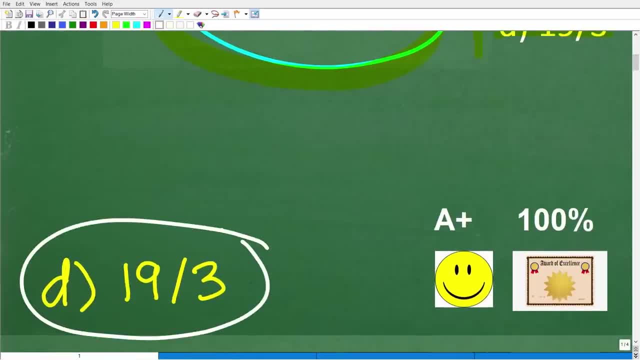 The correct answer is d, 19 over 3.. All right now, if you got this right, you definitely get a happy face, an A+, a 100% and a certificate of excellence for doing a basic calculus integral problem. All right, so what we have here is an integral problem. 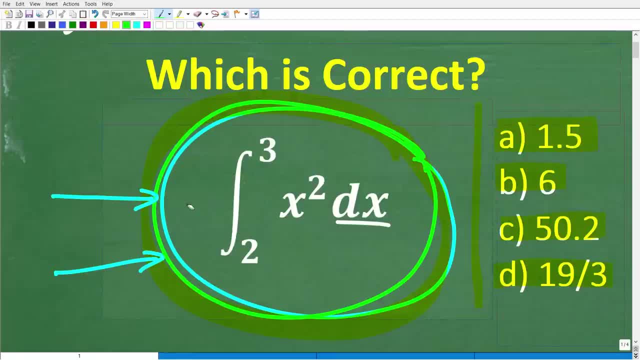 And effectively what we did here was calculate the area. This is really an area problem underneath this curve right here. Now some of you might be saying, hey, Mr YouTube Math Man, I still don't get what's going on. 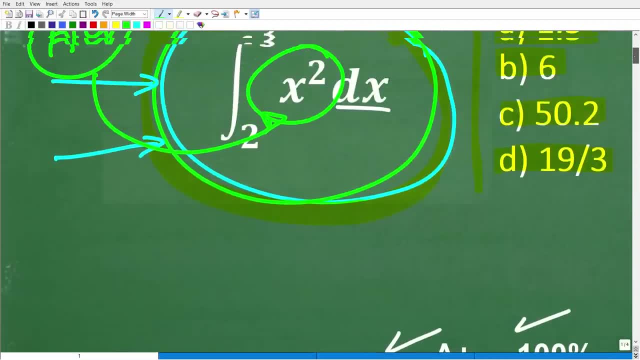 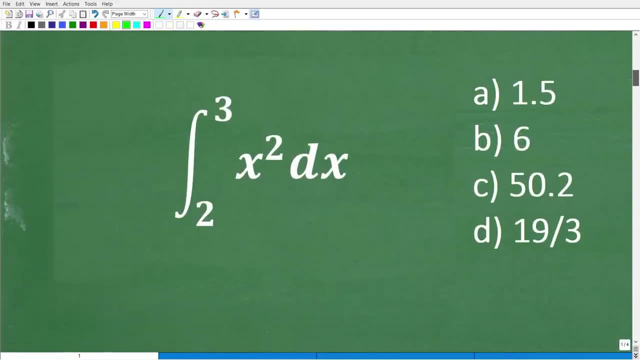 Well, let's go ahead and get into this right now, But for those of you that got this right, that's fantastic. It tells me that you remember some of the calculus that you took way back, whenever that was All right. so what is calculus? 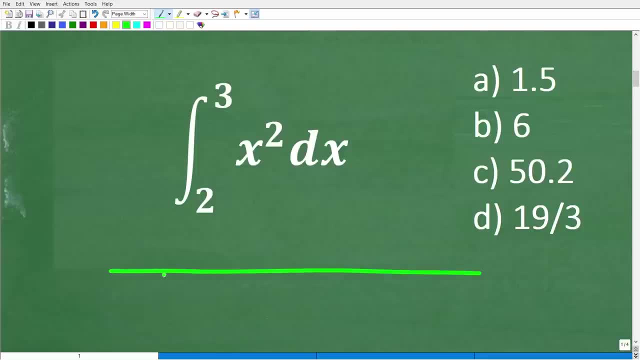 Well, in real kind of basic terms, let's just do something here real quick on when you actually take calculus: who takes calculus and why do you even need calculus? Well, typically let's go back to our high school days. So for most students they take algebra at the 9th grade level and then at the 10th grade level they'll take geometry. 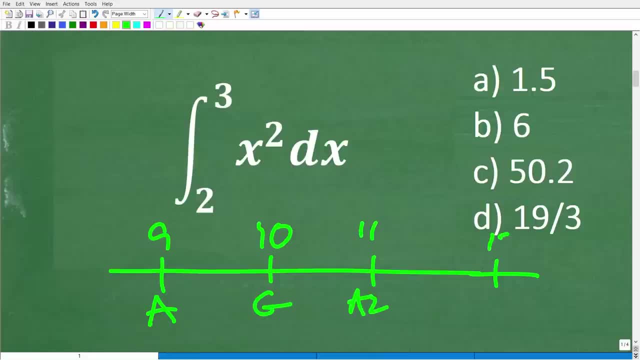 And then 11th grade like algebra 2, and then 12th grade typically like pre-calculus. Some students actually take calculus, So calculus is typically a college level. So calculus is typically a college level math course and not everyone needs to take it. 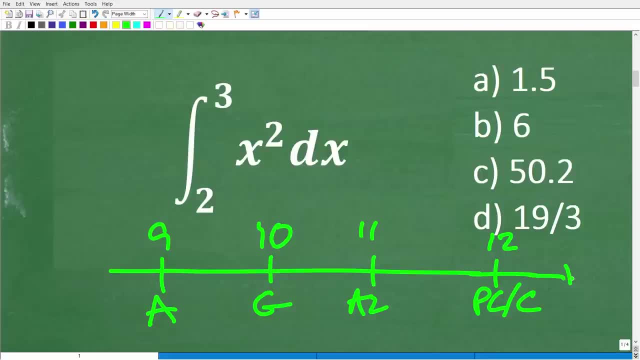 People that generally take calculus are those that are going into some sort of engineering, science, math type of you know major. okay, So you know, if you've never taken calculus, well, you very well may have no need you know to learn calculus. 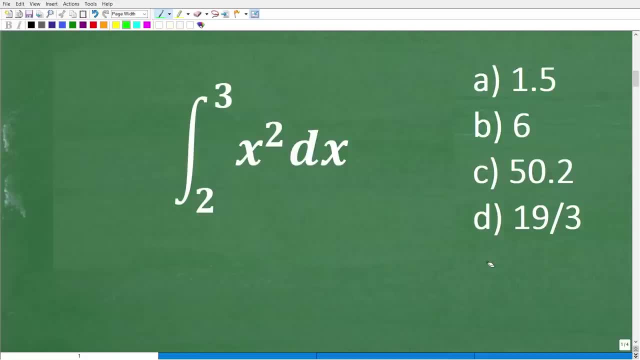 But calculus looks very mysterious. It you know where. you have symbols that you only see in calculus. You don't see these kind of symbols in geometry Or algebra. but remember, math is a language, okay, Like any language. if you don't understand the language, the symbols are going to look kind of funny and crazy. 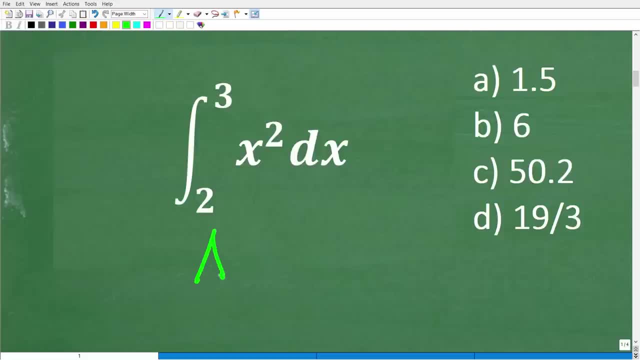 All right, but this particular problem is really an area problem. okay, We're trying to calculate the area here, and what we're going to do is calculate the area that involves this thing right here Now, as I promised, as long as you have some basic math skills and some basic algebra. 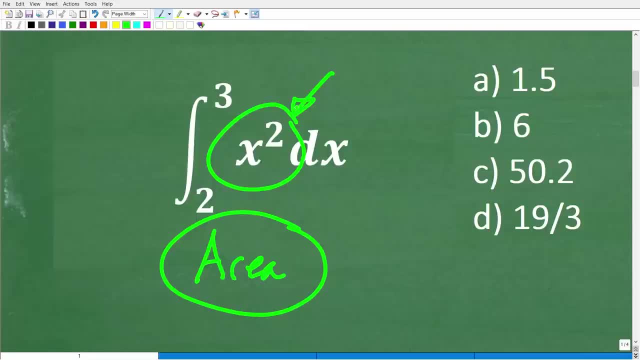 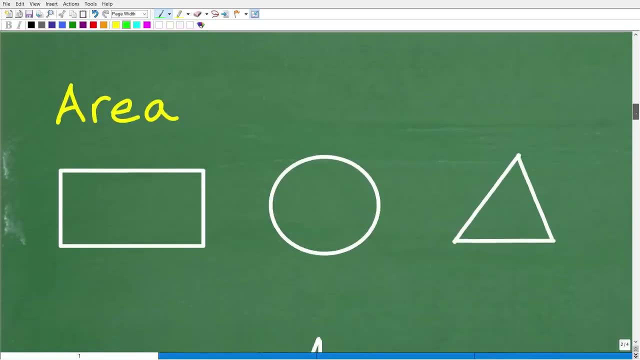 knowledge, you'll be able to understand this. Don't give up, you know if you're lost right now. So let's get into the kind of get into the main concepts of this problem. So we are talking about area, okay. 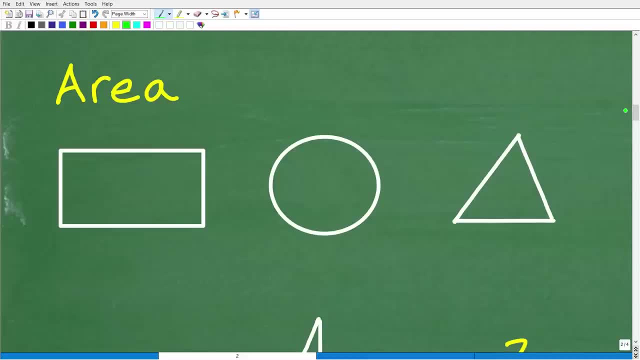 Now, what do I mean by area? Well, let's suppose I said, hey, find the area of this rectangle okay, And you're like, well, I could do that. So we have the length and the width. So how can we find the area of this rectangle? 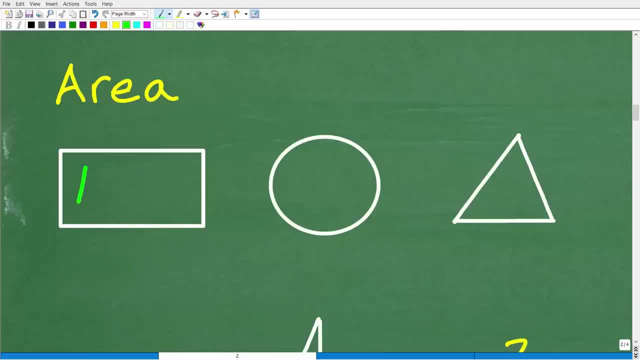 Well, you might be saying to yourself: well, don't, I just need the formula. So yes, indeed, that's right. The area is equal to the length times the width. So if our length was 10 and our width was 5, the area of this rectangle would be 50 square units, right? 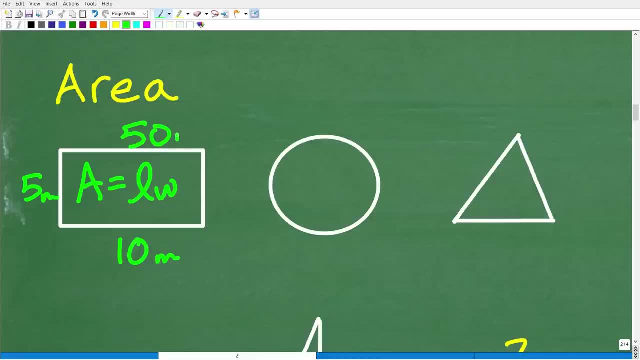 So maybe if this was like meters and this was meters, we would have 50 meters squared, All right. so the main idea here is that to find the area of a figure, as long as we have the formula, we should be okay. 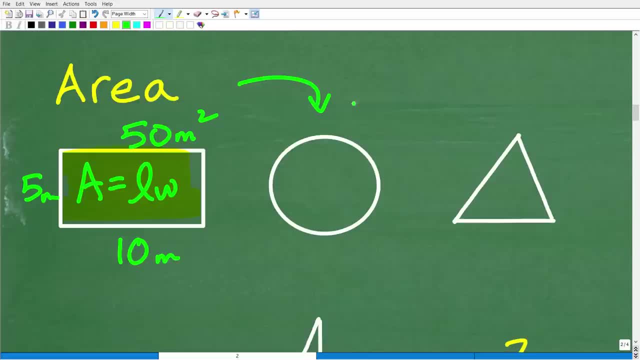 So let's find the area of this circle. Well, we could do that as well, but we need the formula. So the formula for the area of a circle is pi r squared, All right. so how about this triangle? Well, indeed, we can find the area of this triangle, but we need the formula. 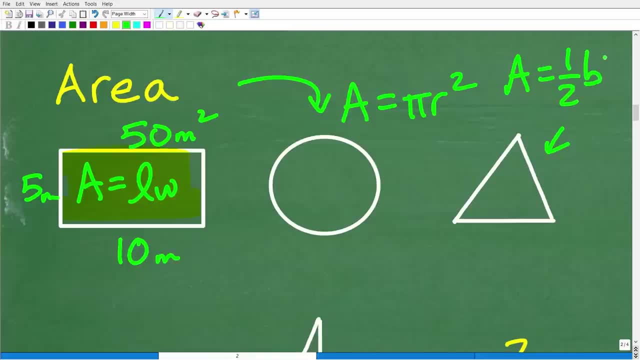 So the area of a triangle is equal to 1 half base times height. So some of you might be saying: well, hey, Mr YouTube Math Man, I can find the area of anything as long as I have the formula. Well, that's pretty good logic. 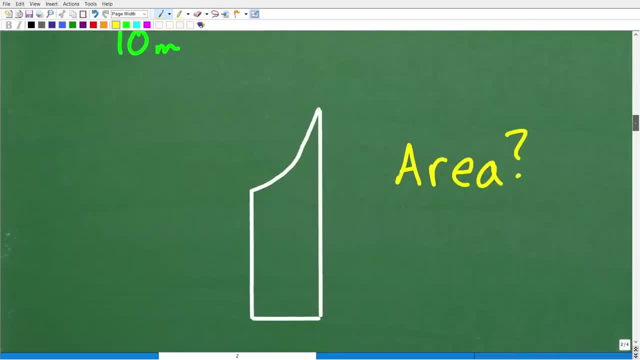 Unfortunately that's not the case, Because what if we had this Crazy looking figure right here? So you might be saying, well, I don't even know what this thing is called, But if you give me the formula, I can calculate the area to this crazy figure right here. 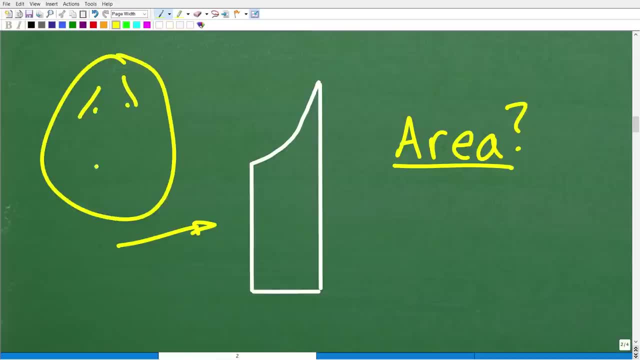 Well, unfortunately, there's no formula that goes to this figure. So you might be saying: well, how are we going to find the area? Well, calculus is going to be our kind of hero And calculus, a huge part of calculus, is helping us find the area and volume of. 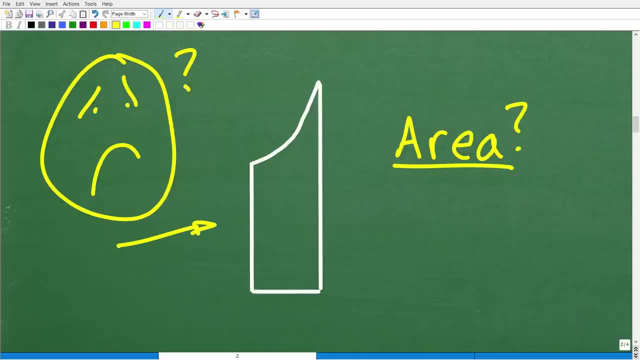 Crazy shapes that we don't have a formula for. So I'm kind of obviously simplifying this. So for those of you that know calculus- or maybe you are a professor of mathematics or like hey, or you're not talking about this and that other thing, 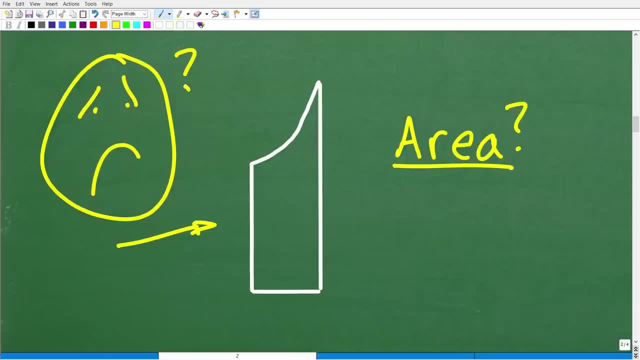 Well, remember, I'm keeping this at a very simple level. So, again, one of the main things, main type of problems that calculus solves for us, is to be able to find the area and volume of shapes and figures that we don't. 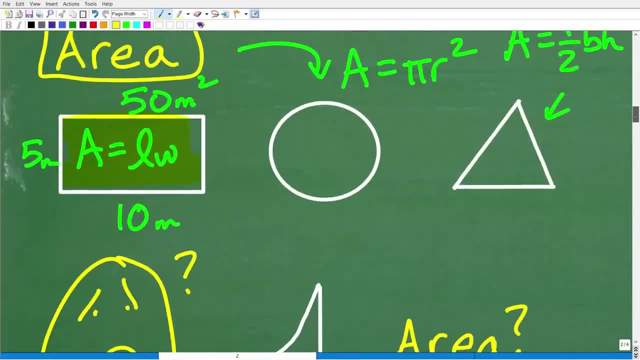 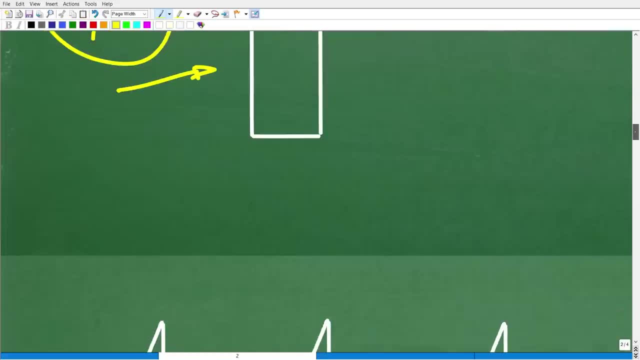 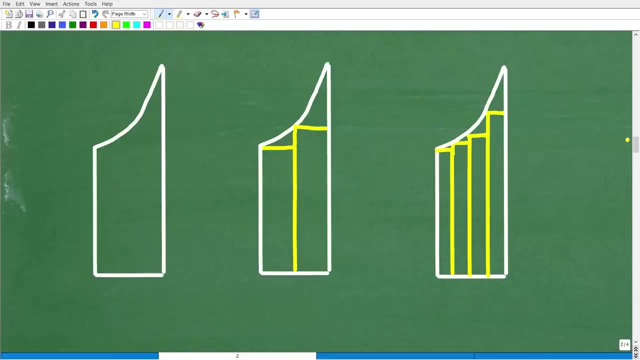 Have a formula for So you know, kind of like nonstandard, you know basic shapes, something like this: How can we find the area of this thing? Well, let's talk about this right now. All right, So one of the main concepts of calculus is, again, to find the area of oddball shapes. 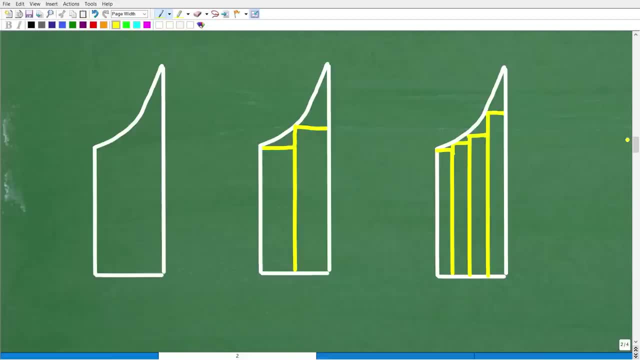 But really well, let's just think about how we can maybe get a pretty good estimate of the area of this figure right here. So some of you might be might say: well, I know how to find The area of a rectangle. 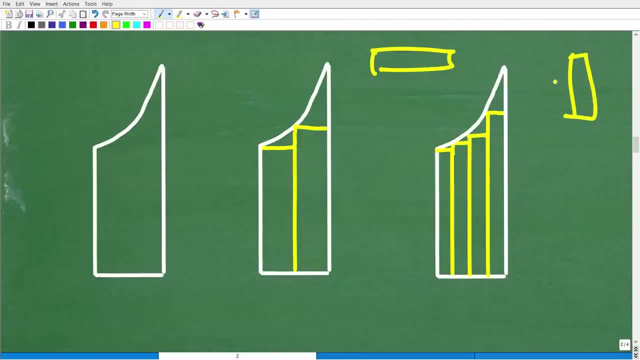 Right. So the area of a rectangle, whether it's this way or this way, is the length times the width. So I could just get a rough estimate of the area of this thing by just going. all right, well, here's the length. 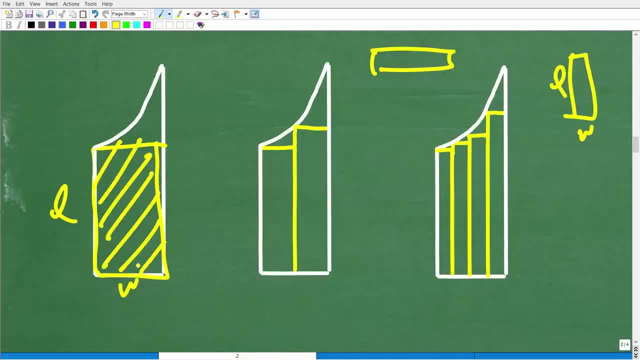 Here's the width. I can at least get this much of this shape Right. The area, We can calculate it out. But you know that's not a great estimate. But what if we use two smaller rectangles? Well, we could kind of go like this: 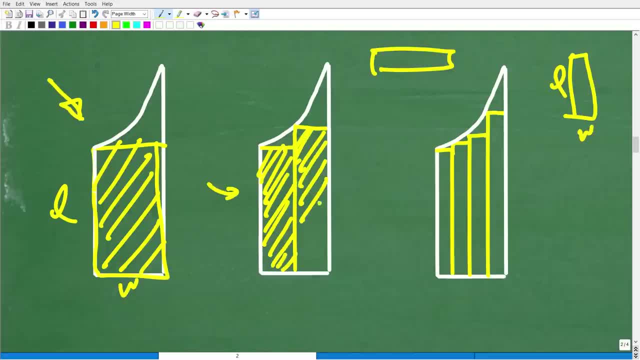 We can find the area of this rectangle And then the area Of this rectangle, And this should give us a better estimation than just using one big rectangle. Well, if we kind of see a pattern here, we could use smaller rectangles to get a better kind of fit for this shape. 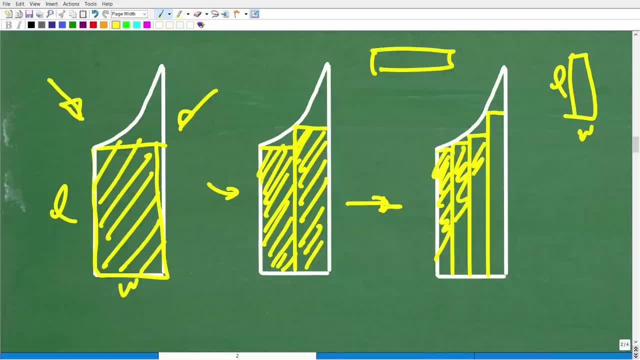 So if we had this little rectangle here and then this one here, and this one here and this one here, we're getting closer and closer to the shape Now if we keep making our rectangles smaller and smaller and smaller and smaller, skinnier and skinnier and skinnier. 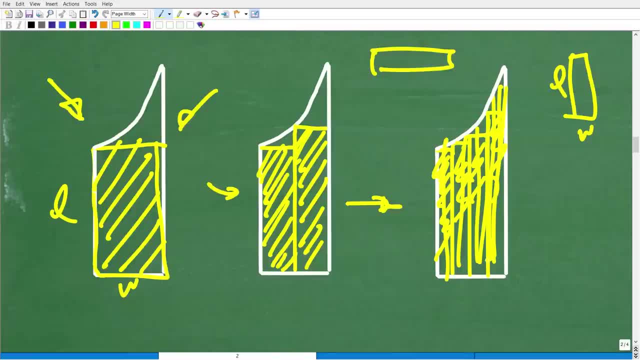 We can literally pretty much get the total area of this figure, And this is the main concept of integration in calculus. Basically, the main idea here is that we're going to take an infinite amount of little, tiny little rectangles, if you will, and we're going to add them up. 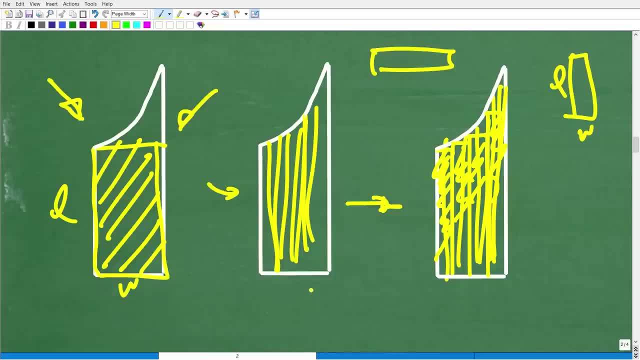 So here's a rectangle, Here's a rectangle, And we're just going to add up an infinite many rectangles And we will have perfectly found the area. Now, of course, from a practical standpoint, that's going to be kind of hard to get the area of all these tiny little rectangles. 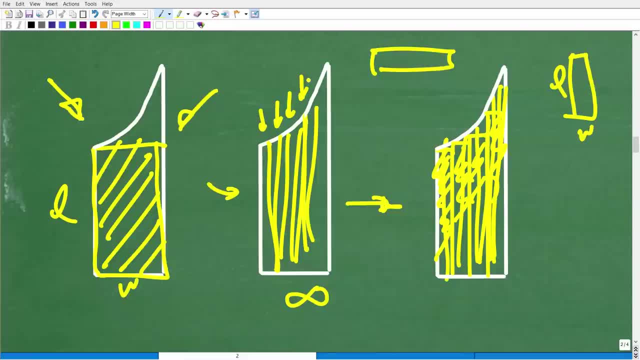 But the main idea of calculus, at least in terms of finding the area of figures, is really finding the area or really finding the sum total of all the areas of these little rectangles. Now, of course, you're going to learn a lot more about this when you actually study calculus. 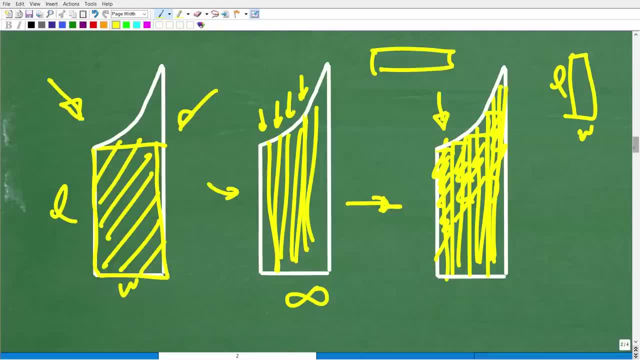 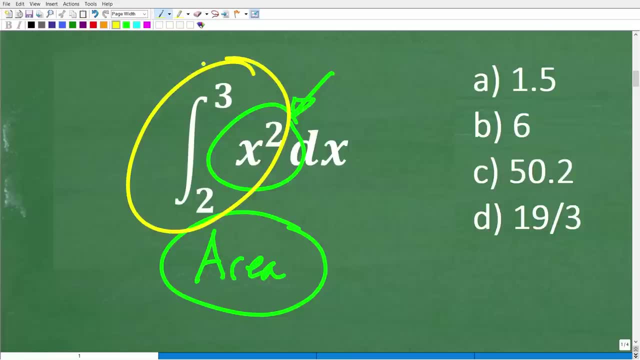 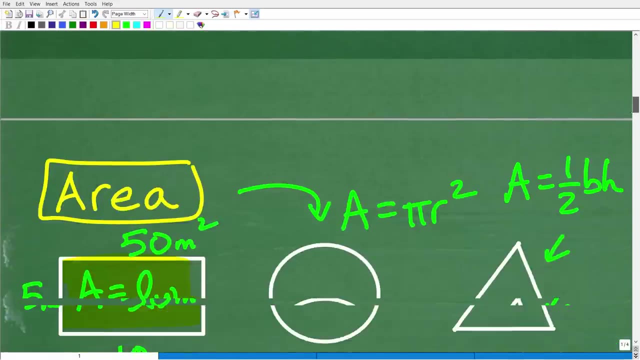 But this is a real kind of main concept of a real Big part of calculus called integration, And that's this symbol right up here. So when you see calculus, this thing right here is called an integral And we're going to talk about what this means in terms of area right now. 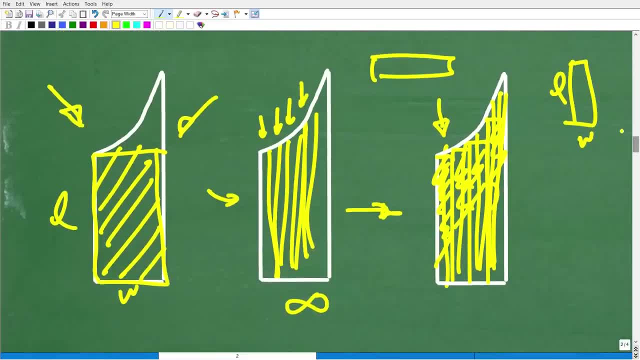 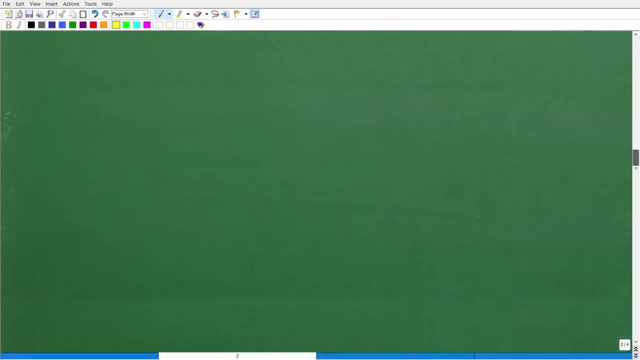 All right. So let's go down here and let's actually do an example problem and find the area of a shape that looks kind of like this. All right, So what we need to do is kind of put that shape on an X- Y plane. 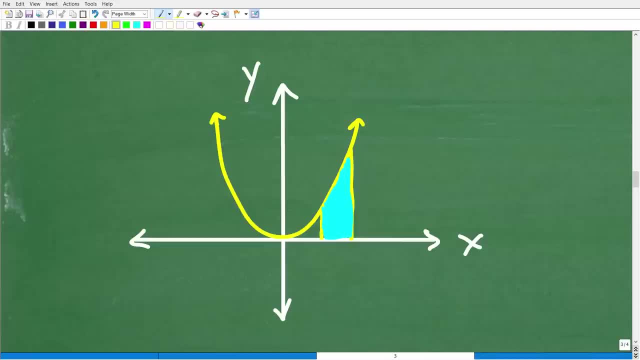 Now, here We're going to give them some basic algebra. So we have an X and Y coordinate system in algebra and we can construct a nice curve right here. Now, the shape that we want to find the area of is this blue shaded shape right here. 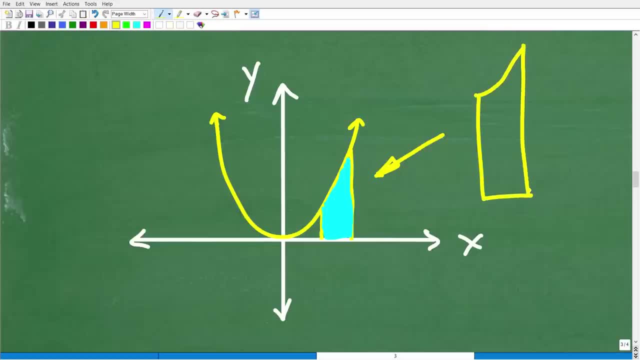 That looks like this shape that we've been talking about with the rectangles. So here, this particular shaded area. we want to find the area of it. So what we need is a description of this. So we're going to take this curve, okay, and then we're going to need some points along the X axis here. 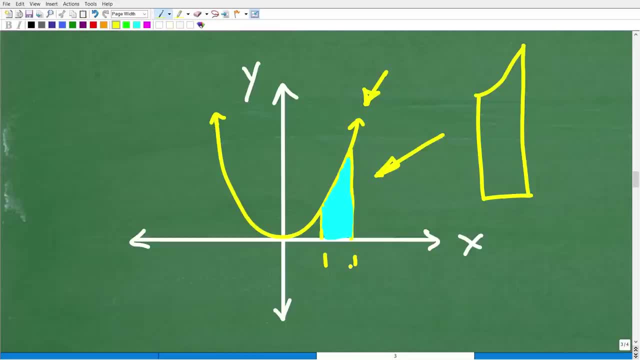 Now, if you don't know much algebra, just stick with me, because you're going to see here that the math involved to actually calculate the area is not that difficult. But let's go ahead and take the next step here and take a look at how we can describe this curve. 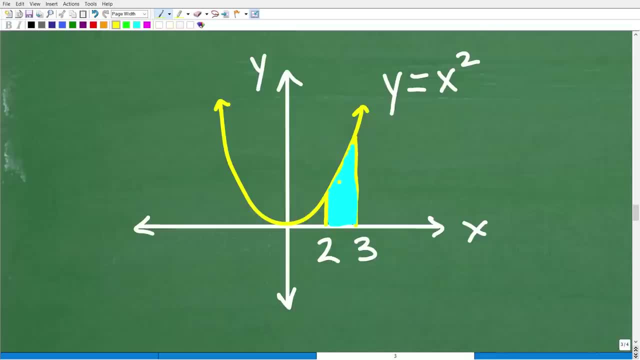 All right. So in algebra we could graph this curve right here by this equation: Y equals X. Okay, So Y equals X. squared is this U-shaped graph. This is called a parabola, So it goes like: so: Now, along the X and Y axis, there's these points. 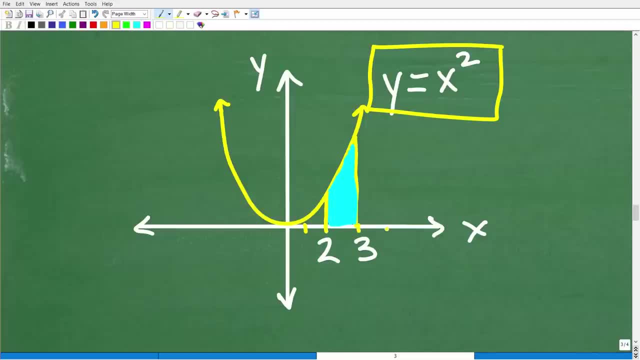 Okay. So in other words, it's just a number line. So we have 1,, 2,, here's 3,, and there's 4,, there's 5. And then we can go positive 1,, 2,, 3,, 4,, on and on and on. 1,, 2,, 3,, 4, in all these directions. 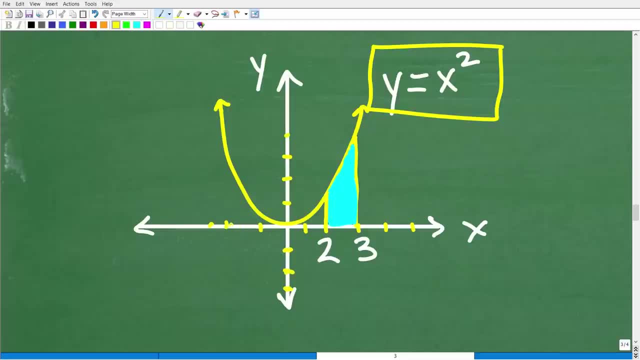 This is negative 1,. actually, This is negative 1, negative 2, negative 3, negative 1, negative 2, negative 3.. As long as you have some basic idea of algebra, this should look somewhat familiar to you. 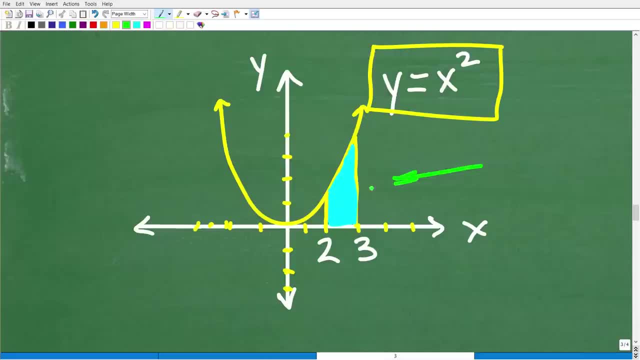 So remember, the objective here is to find the area of this part underneath this curve described as: Y equals X squared. This is the equation to this graph. Now you can actually construct the points on this graph by creating a table, an XY table. 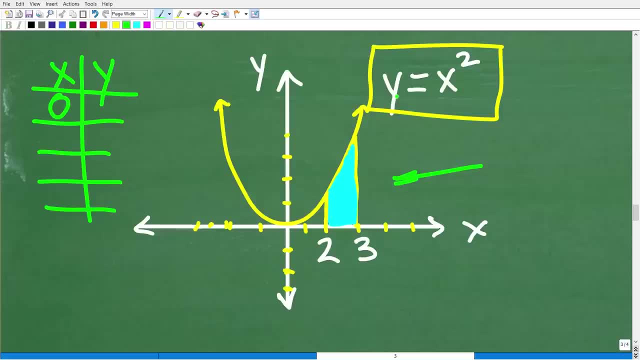 So when X is 0, okay. what is Y equal to? Okay At Y. if I know what X is equal to, I would just plug in a 0 for X. So 0 squared is our Y, So that's 0, 0.. 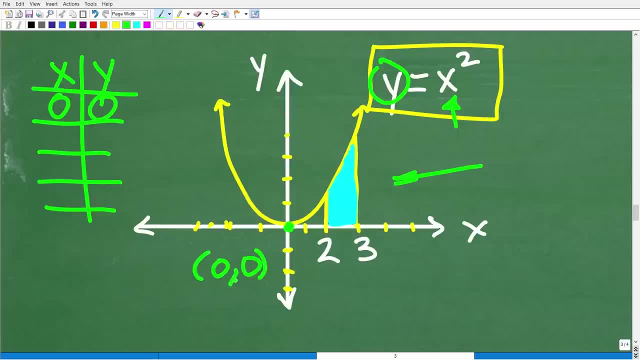 So that's the point right here: 0, 0.. All right, When X is 1,, what is Y? Well, let's plug in 1 for X. Well, 1 squared is 1.. So 1, 1 is on this graph. 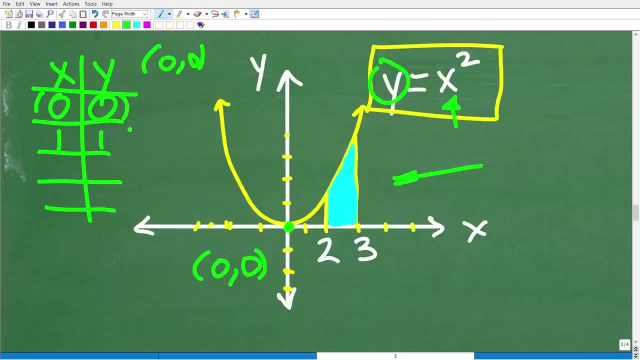 These are actually what we call coordinates. 0, 0 is a point on this curve. 1, 1 is a point on this curve. So here would be 1, and let's say that would be the point 1, 1.. 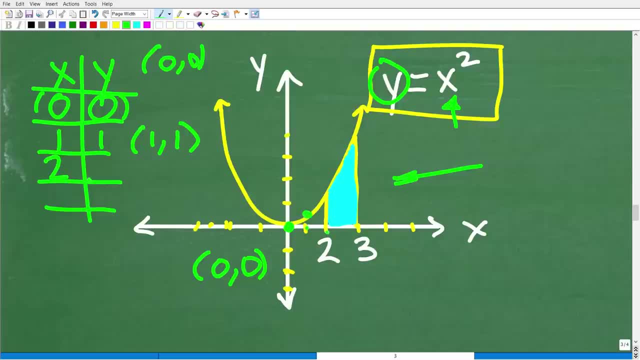 All right. So when X is 2, what is Y? So we're going to plug in a 2 for X. So 2 squared is 4.. So Y is 4 when X is 2.. So the point 2, 4 is on this curve. 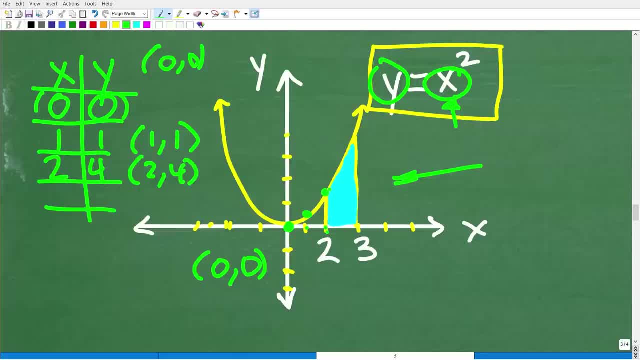 So here's 2, and this would be like 2, 4.. So you can kind of basically play, connect the dots and just, you know, list out a bunch of X points here, and then you can kind of construct this curve. 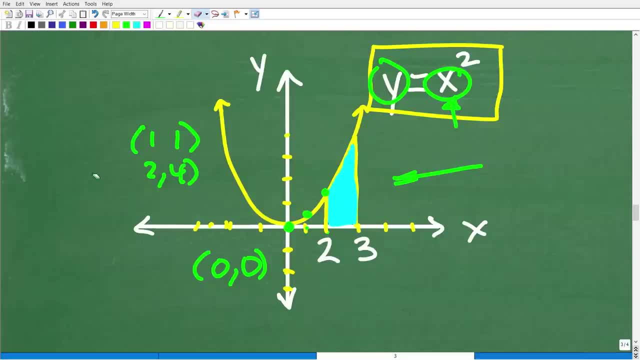 So you know we're not talking about too difficult of mathematics here and hopefully you are with me, Okay. so here is where we're at. Y equals X squared is the equation that describes this curve, and we want to find the area underneath this curve, bounded by the X axis. 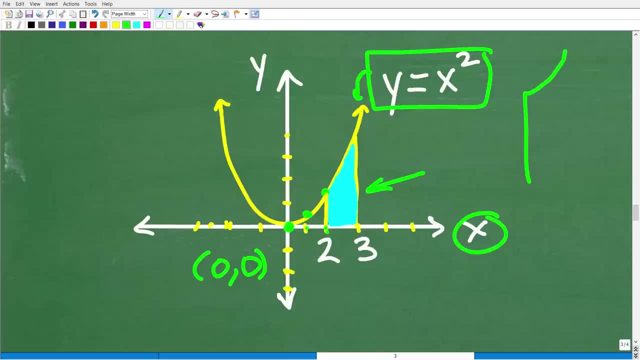 In other words, this shape right here. So this is what we want to do: We want to find the area of this shape and we already discussed how we could kind of construct some rectangles to actually figure this out. But we're going to use calculus now to figure out the area underneath this curve. 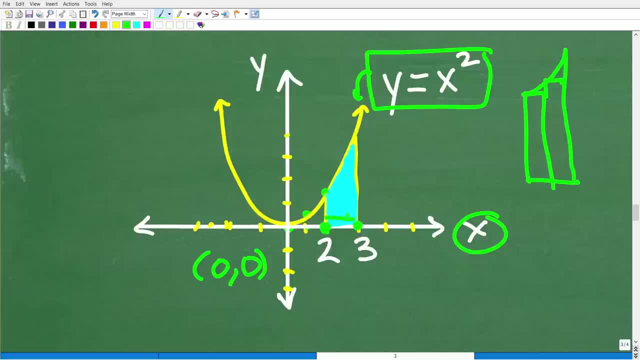 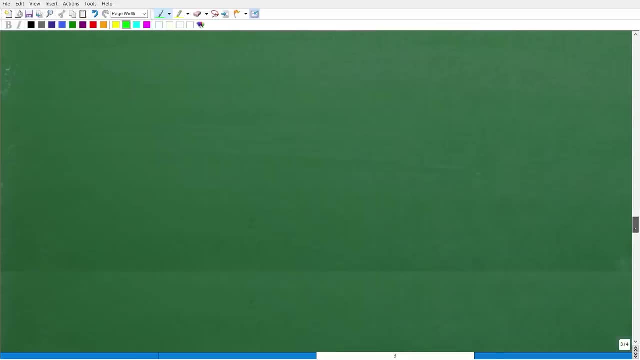 from 2 to 3 on the X axis. Okay, All right. So if you're with me so far, let's actually write some calculus here, and this is the way it would look. All right, So here is calculus. So calculus is going to say: this little long thing right here is called an integral. 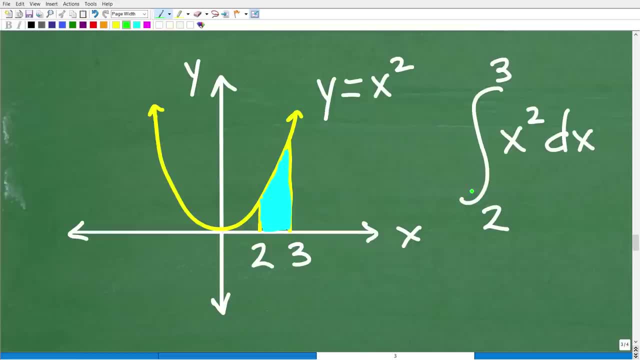 Technically it's called an elongated S, but you don't need to know that. But basically it's the sum, or, effectively, what we're trying to do here is add up. You can think of this thing as add up all the rectangles between 2 to 3.. 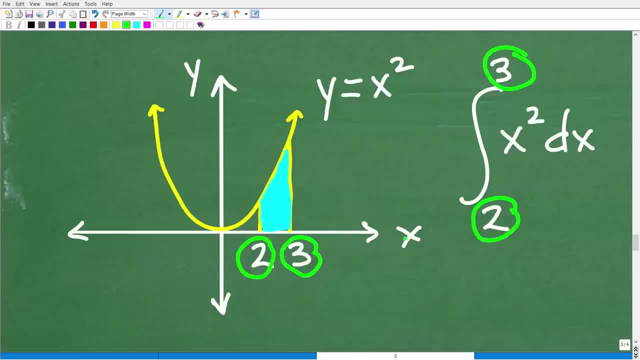 Start at 2 and go to 3.. We're going to add up all the rectangles, the little skinny rectangles from 2 to 3, underneath the curve X squared. Okay, So that's what this calculus notation means. Let me go and repeat that one more time. 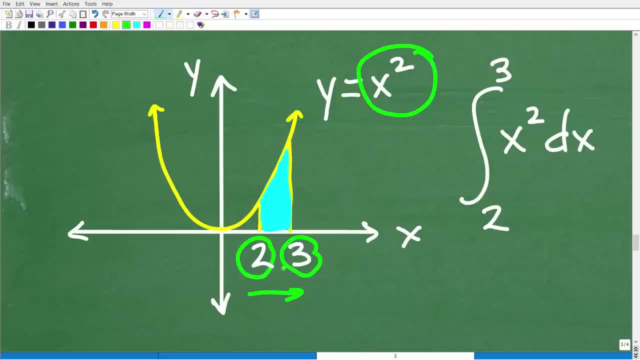 So it says: add up, okay, all the rectangles underneath this curve, X squared, start from 2 and go to 3,. okay, on the X axis. And when we add up all the infinitely small rectangles, we will have calculated the area of this shape right here, and that is the goal. 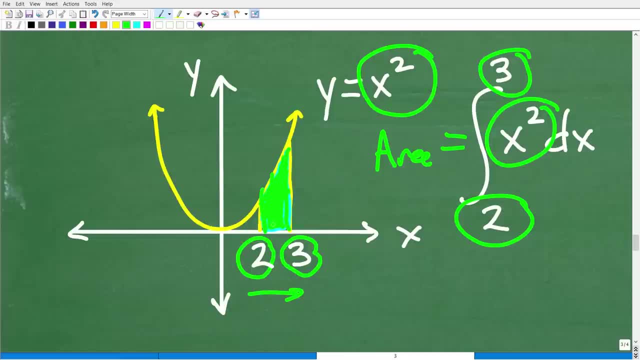 All right. So if you're with me so far, now some of you might be saying: well, I kind of get what you're saying. Well, this video is intended to be a simple introduction to calculus. You'll learn a lot more about this when you actually take the subject. 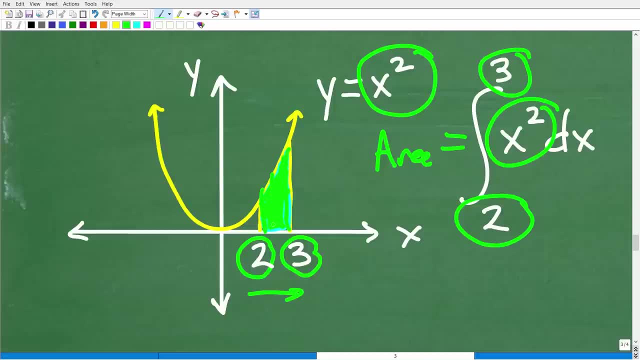 but at least you'll have some sort of, some sort of appreciation of why we need calculus and some sort of understanding, a basic understanding of what this notation is saying, okay, this integral notation, and this is a very common, you know, symbol in calculus. 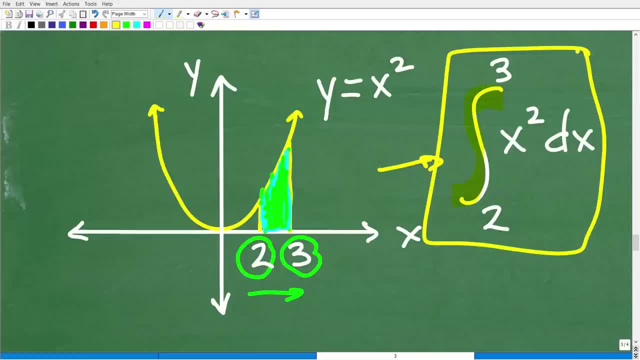 All right. So now what we need to do is actually calculate the area, and again, we're not going to need to know much math. We're going to be talking about some basic fractions, really in order to calculate the area. All right. 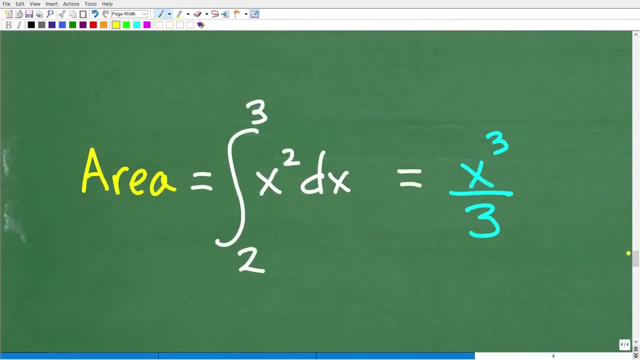 So let's go ahead and get into that right now. So the area underneath that curve, okay, and again we're talking about this little crazy shape, right there is going to be equal to this thing right here. this integral from 2 to 3, x squared dx. 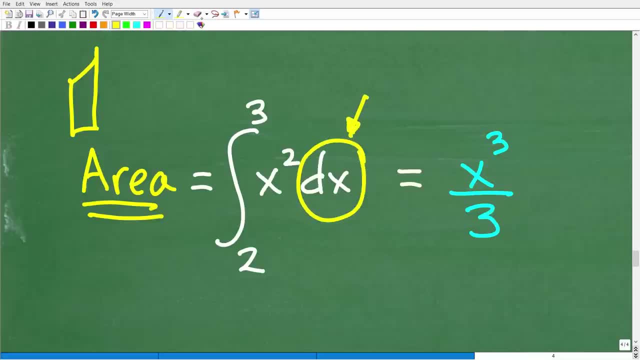 Now some of you might be saying, hey, Mr YouTube, Math Man, what does this dx thing stand for? Well, that's for another video and that's really not so important at this level of calculus. This is important, obviously. 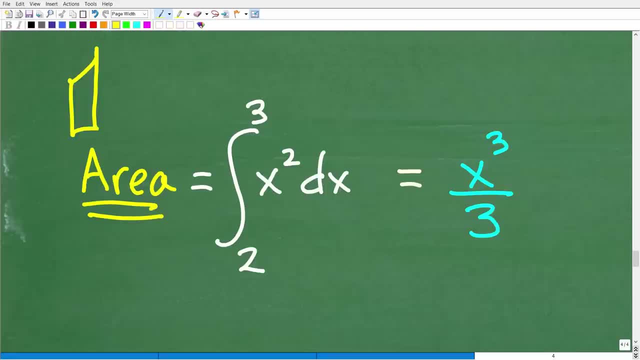 for those of you that will actually take the subject, but for what we're doing here we can kind of disregard that, dx, but that is part of the notation to actually write this problem out. Okay, so we need to figure out what this thing is equal to. 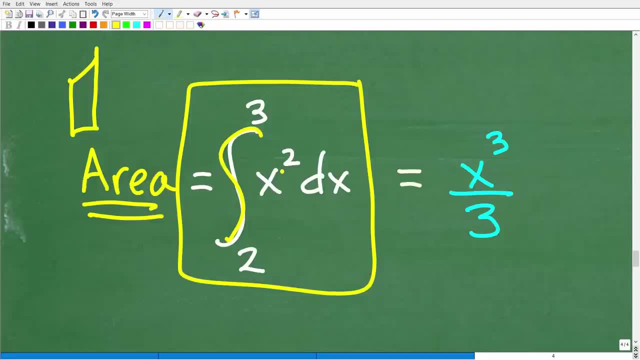 this integral x squared. All right, so I have the answer right here. It's x cubed over 3.. Now let's talk about how we do this. okay, All right, let's pay attention to this x squared and we're going to do this integral of x squared. 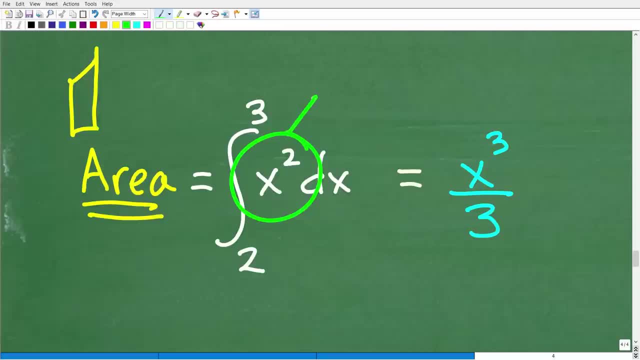 and the answer is this: Okay, All we do, let's focus in on the x squared right here. Okay, here's x squared. is we're going to add 1. There's a rule? okay, There's actually a lot of rules in calculus. 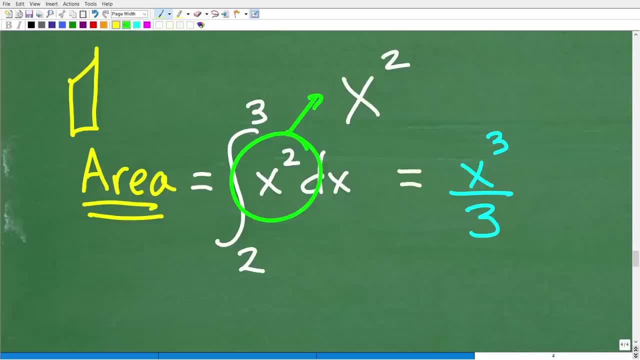 They're not that difficult to follow. It's just a bunch of rules you need to learn. So in this particular situation, the rule says: just add 1 to the exponent. So here this is 2, okay, So we're going to add 1 to 2, all right. 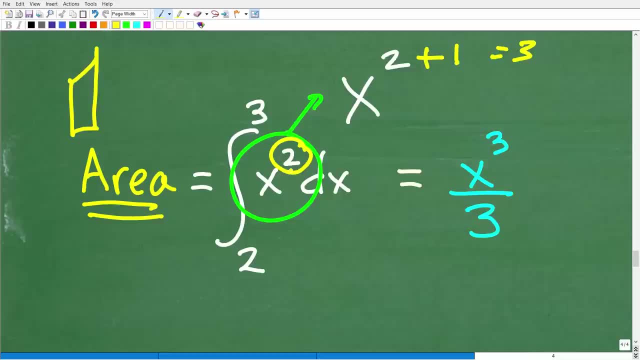 So 2 plus 1 is what? Well, that's 3.. So the rule is: add 1 to whatever, whatever this power is in this exponent. So that's 2.. So we're going to get x to the third power. 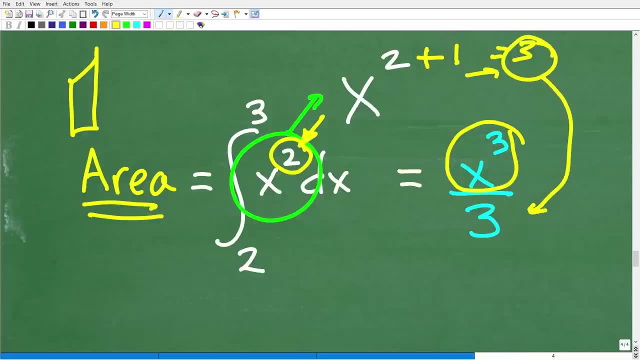 Now, whatever, the answer is the exponent divide by that. okay, So that is what the rule says. So we have x cubed divided by 3.. So once again, let me go ahead and explain this. We need to do this little integral here. 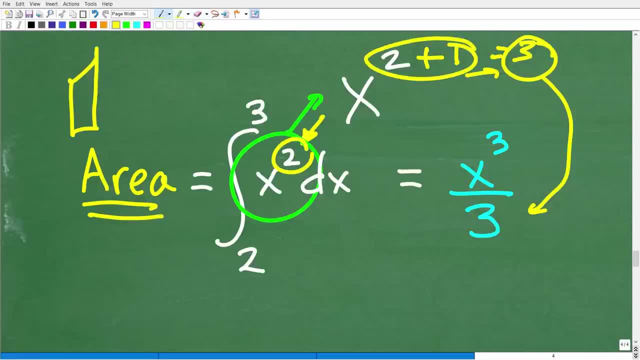 So we have x squared. So, once again, we're just going to add 1 to the power, whatever that's equal to. we're going to divide the entire thing by All right, So we're going to end up with x squared. 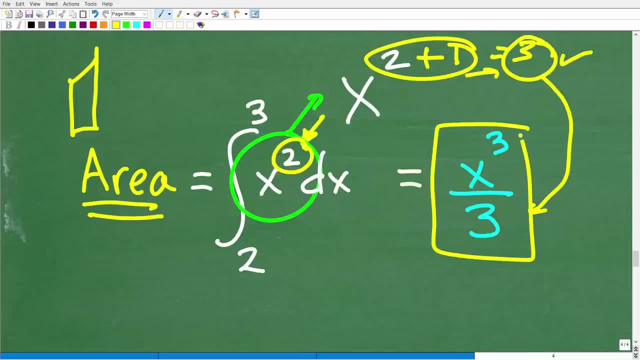 So we're going to end up with x squared. So we're going to end up with x squared. So we're going to end up with x to the third power. We're going to divide by 3, because that's what we got up here. 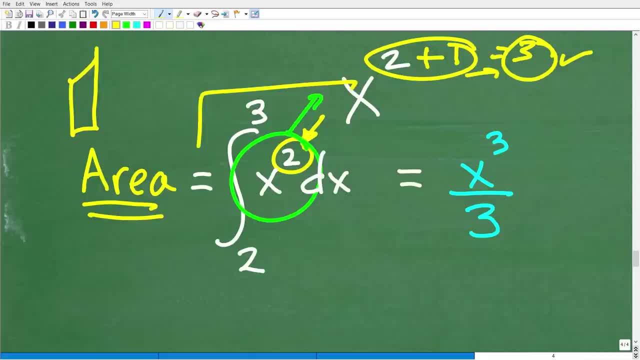 All right, So we are almost there. So all of this. okay, we haven't even calculated the area yet, but we did take care of this integral part. This integral x squared is equal to x cubed over 3.. 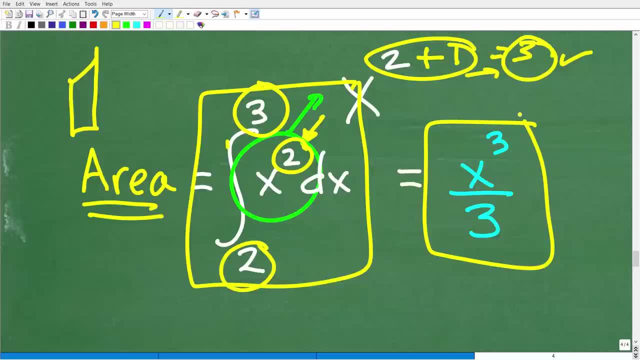 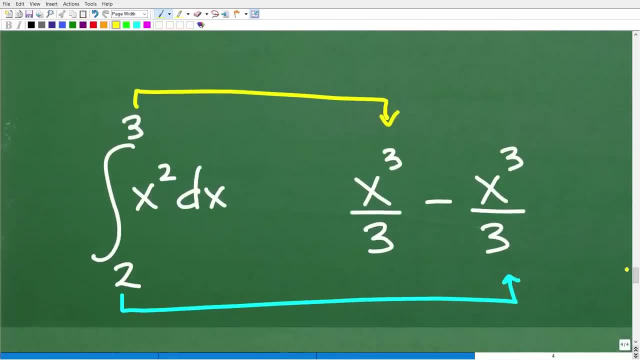 Now we can actually calculate the specific area to this shape, All right, So let's go ahead and do that right now, And what we're going to do is the following: So here is our integral right, which means add up all those skinny little rectangles. 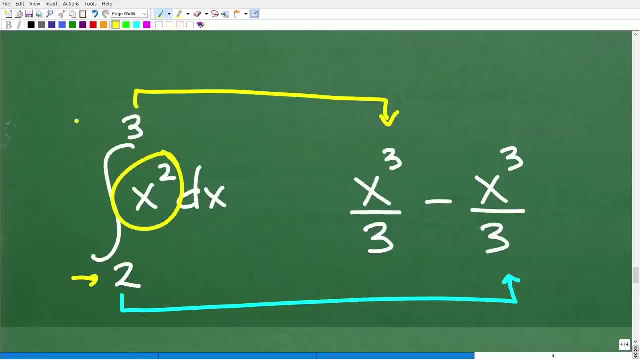 or find the area underneath this curve from 2 to 3.. And what we're going to do is take our answer to doing this integral, which is x cubed over 3, and we're going to subtract it from itself. Okay, x cubed over 3 minus x cubed over 3.. 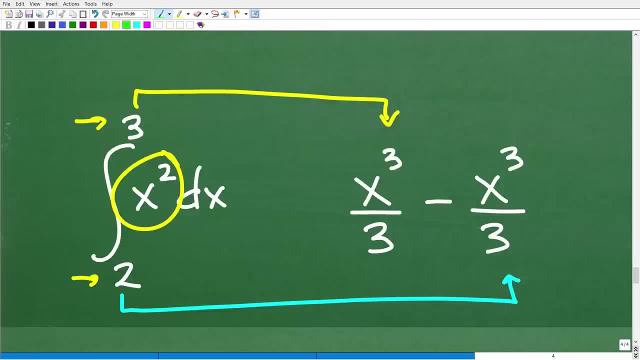 This is how we do this in calculus. Whatever we did here, we're going to actually subtract it from itself, but we're going to plug in. We're going to plug in the top number on this integral, right here. Okay, so we're going to replace this x with 3 on this first one. 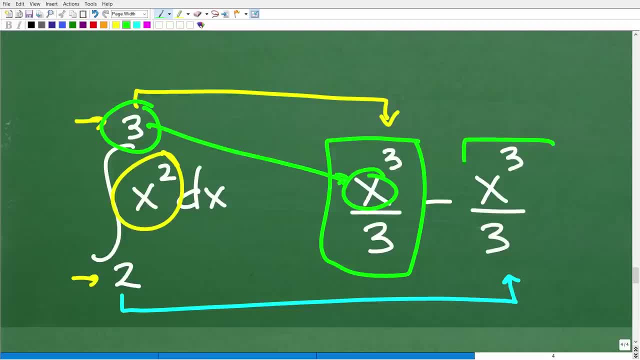 Okay, so this x is going to get replaced with a 3.. And then on this second one, this x is going to be replaced with a 2. And when we do this number crunching, we will have actually calculated the area of this shape. 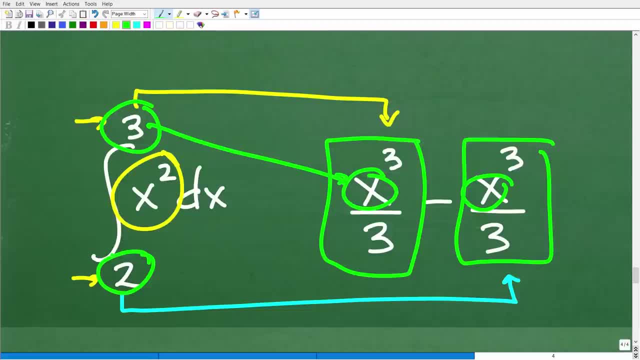 Again, I'm not doing 2,, you know, and I'm not doing a lot of advanced algebra or anything, And you're going to see here where what we're really going to be doing is just a bunch of fraction work. So as long as, again, if you have some basic math skills, 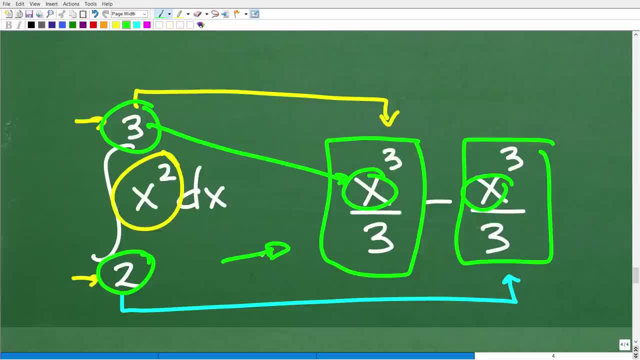 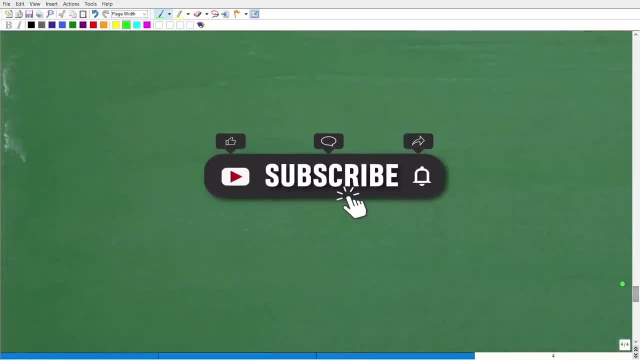 and basic algebra knowledge, you should be able to kind of follow along on what's going on in terms of this calculus problem. Okay, so let's go ahead and do that number crunching. But before we do that, let me go ahead and have you do this. 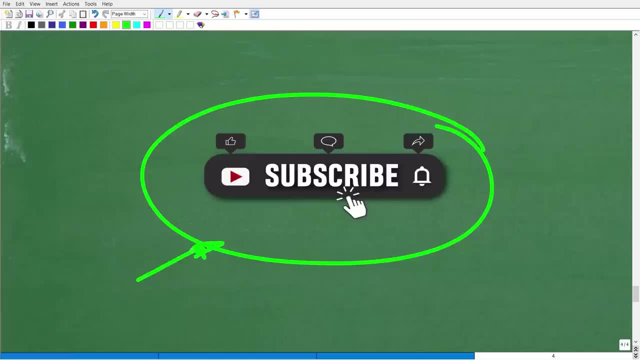 And that is to quickly subscribe to my YouTube channel. Now, putting these videos together, you know, I really try to think about how can I explain concepts that seem very complicated in a way where people kind of appreciate, like and understand, Because oftentimes math, especially advanced math, 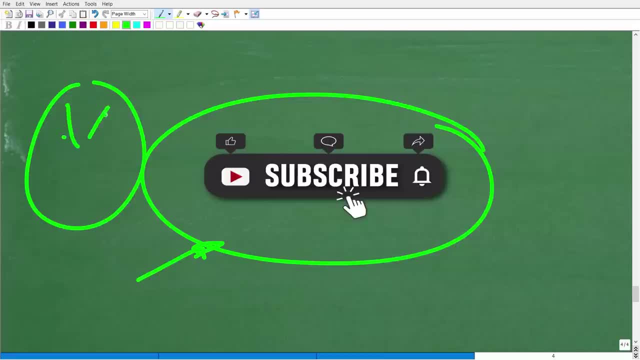 is just very mysterious to people. They get you know, too intimidated by it. They're like: hey, Mr YouTube, Math Man, there's no way I'll be able to understand. I'm not that smart in math. Well no, you can do calculus. 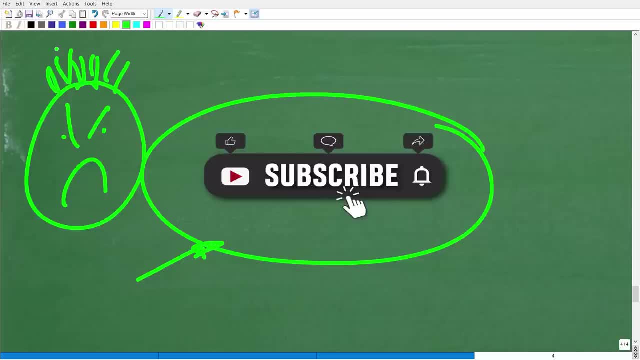 So if you ever wanted to do calculus or learn calculus, let's say you certainly can. all right, It has nothing to do whether you're smart enough. I'm telling you right now you're definitely capable enough And the concepts you know, once you kind of have a basic sense. 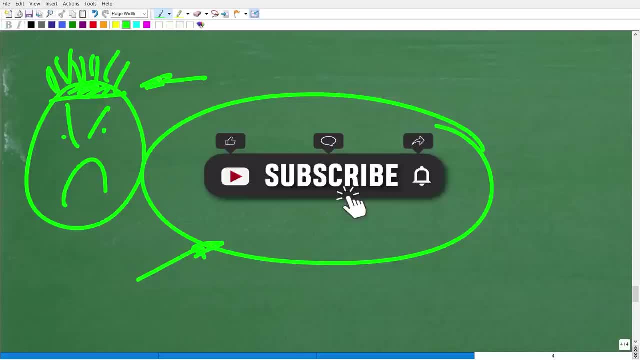 of what the subject is about. I think that gives people maybe more confidence that they can actually learn this stuff- And you absolutely can, But it is a journey. There is a lot that you really need to know before you actually take a real calculus course. 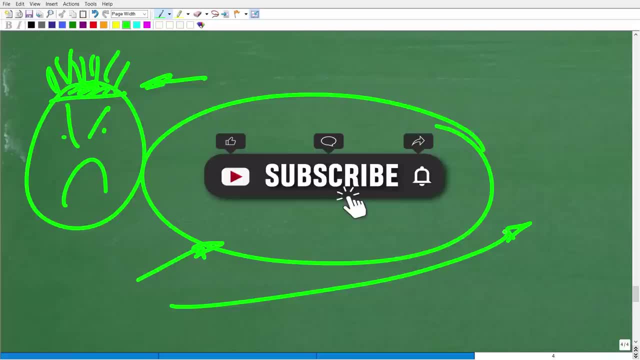 Now, if you're interested in calculus and you want to get ready for that subject, the most advanced math course that I offer is pre-calculus, And you definitely need to master all of that before you actually take a full calculus course. But if you're interested in my pre-calculus course, 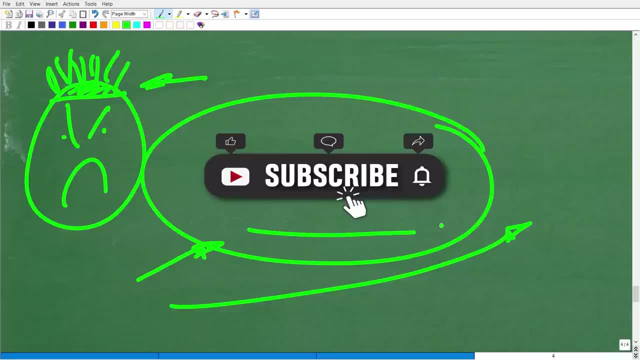 you can check that out. You can check out my full pre-calc course by following the link in the description. But if you just want to simply rebuild your math skills, check out my math skills rebuilder course. Or if you need help in you know, geometry or whatnot. 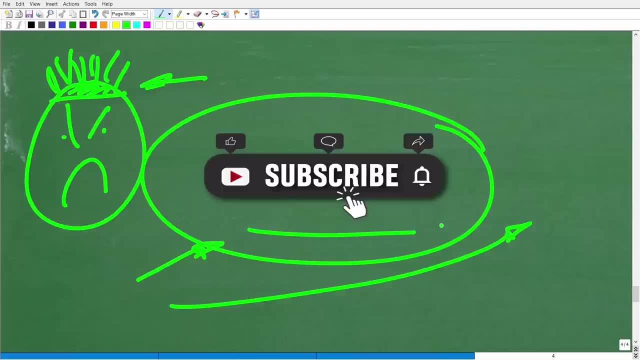 you'll find a lot of links in the description to various courses. Also, I have a ton of content On my YouTube channel that can help you out, But I need your help on YouTube. So certainly, you know, by you subscribing to my channel. 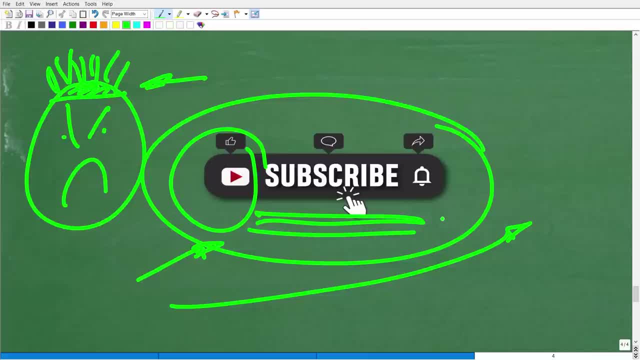 that's a big deal. That's why I'm stopping this video and asking for your help, And if you're going to do that, make sure to hit that notification bell as well, so you can get my latest videos. All right, so let's go ahead and finish up this problem. 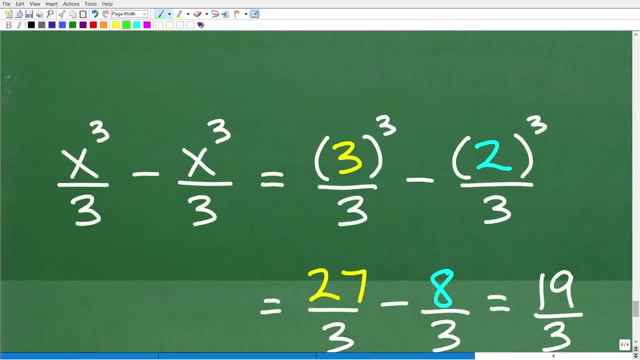 so we can get the actual area. Okay, so here is our x cubed over 3 minus x cubed over 3.. Remember, we're going to plug in that top number on the integral, which was 3 in this first. 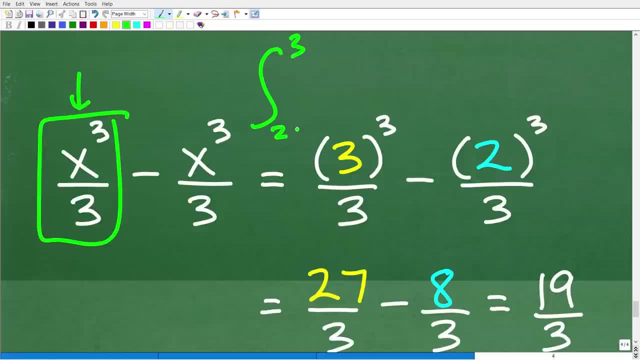 x cubed and then our bottom number, which is 2, we're going to plug it in on this second one. So here is the setup. So we have 3 cubed over 3 minus 2 cubed over 3.. 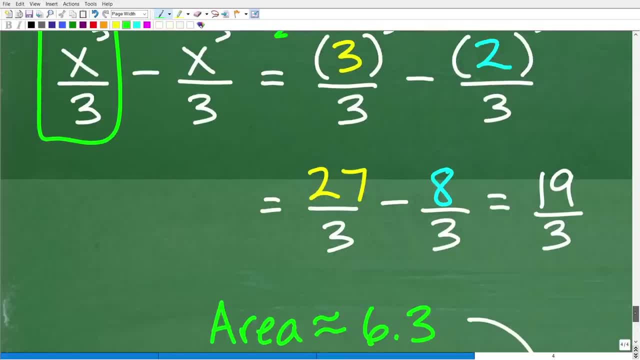 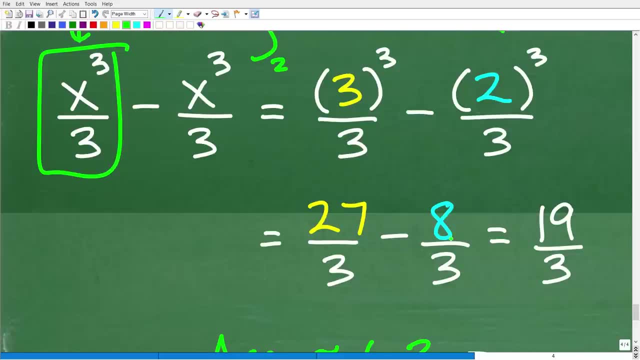 And let's go ahead and do the number crunching right now. So 3 cubed is what, That's 27,, 3 times 3 times 3.. So 27 over 3 minus 2 cubed, which is 8,. 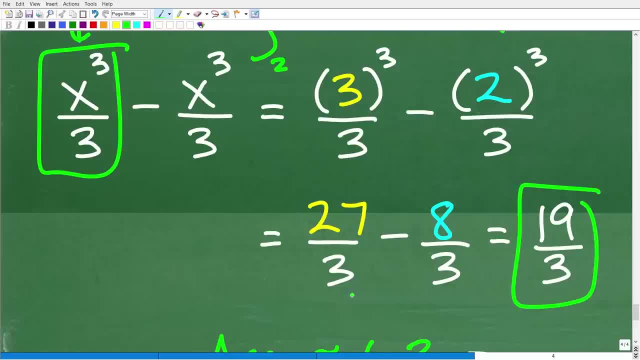 2 times 2 times 2 over 3.. So when we do this simple fraction subtraction problem, we have 19 over 3.. Which is the answer. But if you take 19 and divide it by 3, effectively what you have is 6.3.. 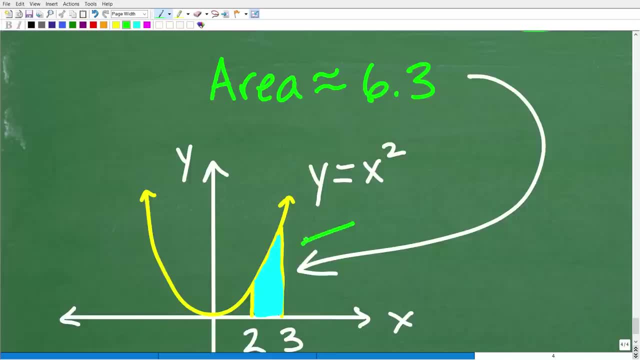 And that is the answer. So that's the actual area of this little shape underneath this curve, x squared. So that is a precise area: 19 over 3.. And some of you might be saying, wow, that's kind of fascinating. 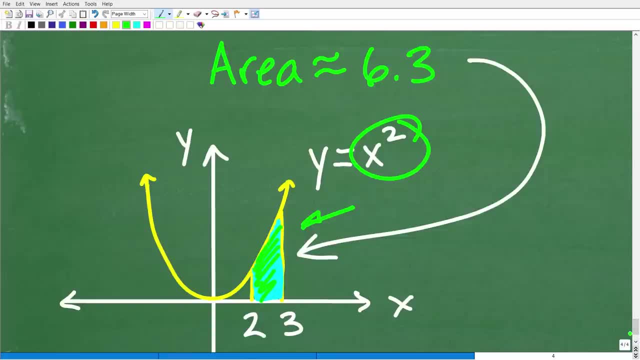 And hopefully you weren't overly, let me just say it this way- you weren't overwhelmed with the amount of math to actually calculate the area of this crazy looking shape underneath this curve. And that was kind of the main idea of this video was not to overwhelm you with all this advanced math. 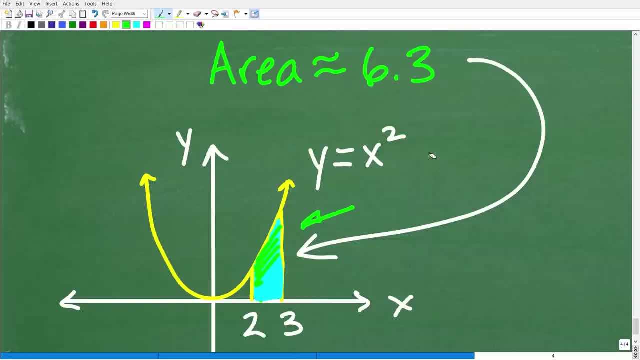 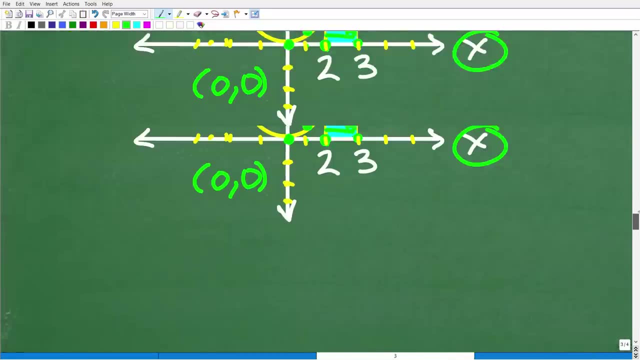 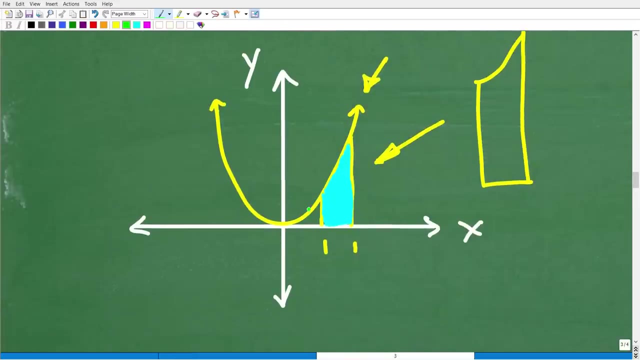 I tried to explain this in a way where pretty much anyone can understand, even if you didn't understand it perfectly. hopefully you have some sort of sense of what calculus is about, at least a big part of calculus, which, once again, is to find the area and volume of shapes. 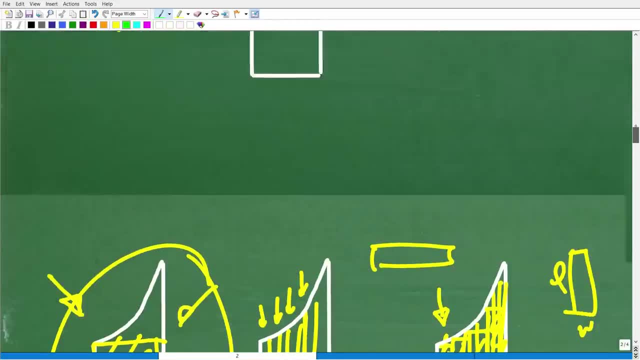 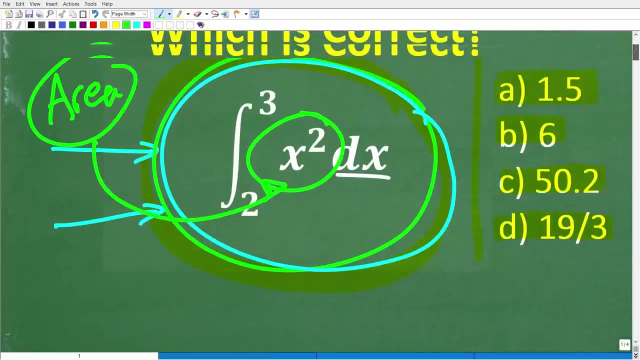 where we don't have lovely little simple formulas for, like, a rectangle, a square, a circle, a triangle, etc. etc. Okay, so, once again in mathematics you're going to come across symbols and notation that, if you don't know what they mean, 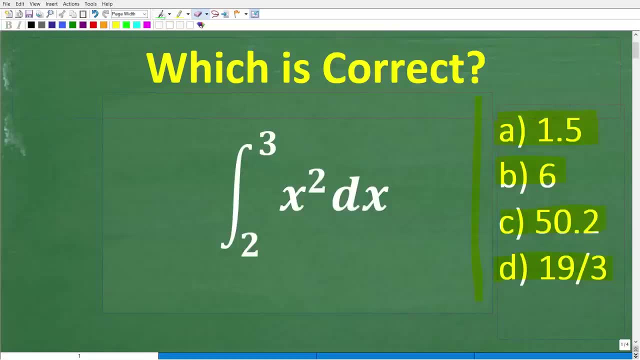 they're going to tend to intimidate you in the sense that you're going to be like: oh, this is too hard, I'll never be able to figure it out. Well, what you have to do is just take on these new symbols that you encounter in math, one at a time. 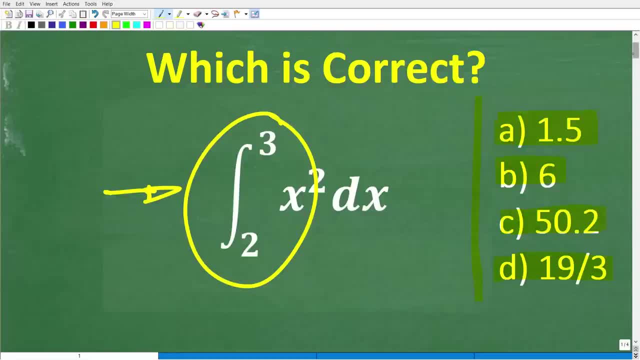 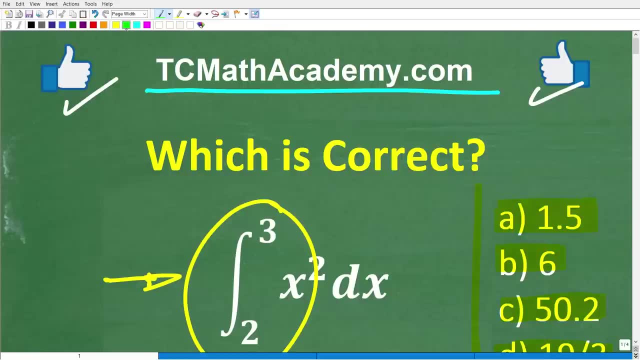 And more often than not, you're going to find out that they're really not that bad, Okay. so if this video was interesting or if some way it inspired you to maybe want to learn calculus, make sure to like and subscribe. And with that being said, 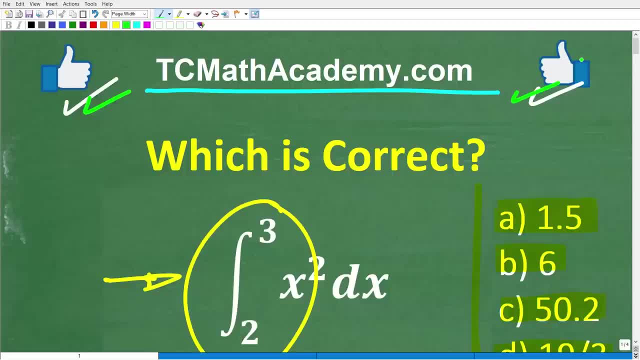 I definitely wish you all the best in your math adventures. Thank you for your time and have a great day.